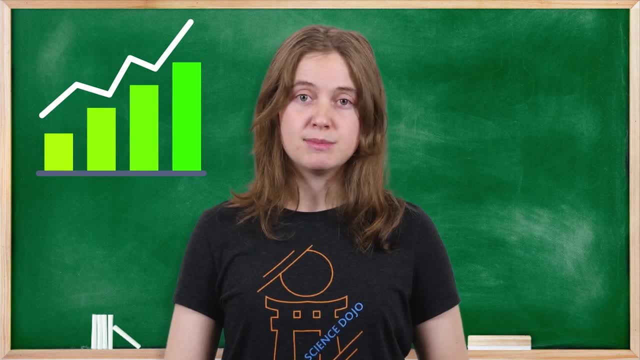 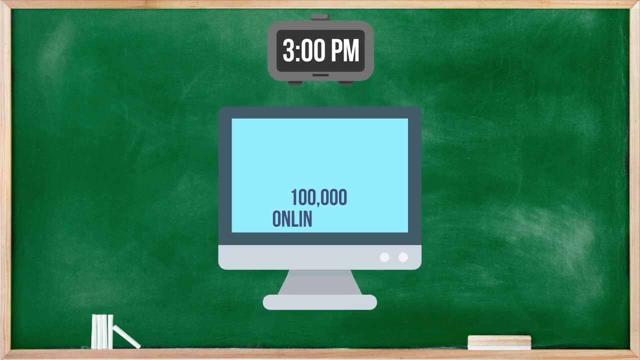 continue, but a time series forecast can give us a better estimate or figure for how much it could continue. For example, given this time of day, a time series model predicts 100,000 people to log in online. You might have known there would be a lot of people online, but now you can plan. 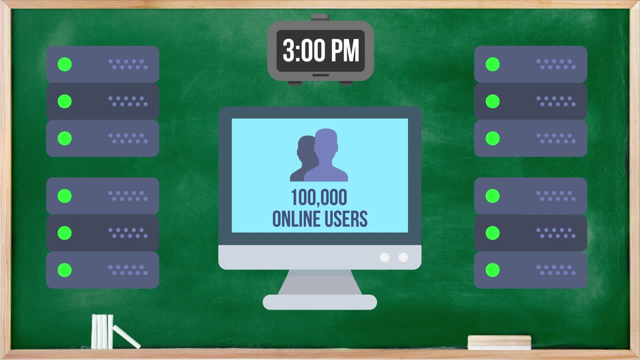 for how many additional servers and infrastructure you need for your online platform, based on how many online users are predicted. You'd only use those servers for that particular time of day, switching them off for the rest of the day, when you don't need them, to save a bit of money. Or it could be that the model predicts. 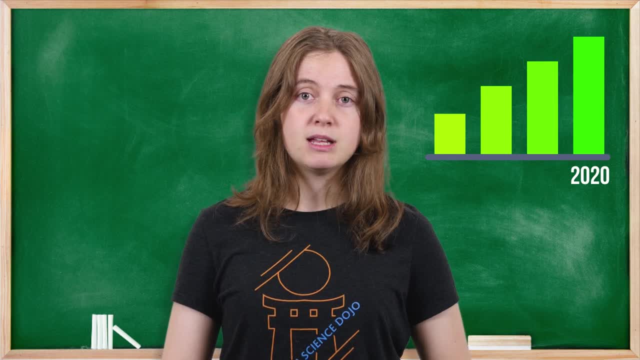 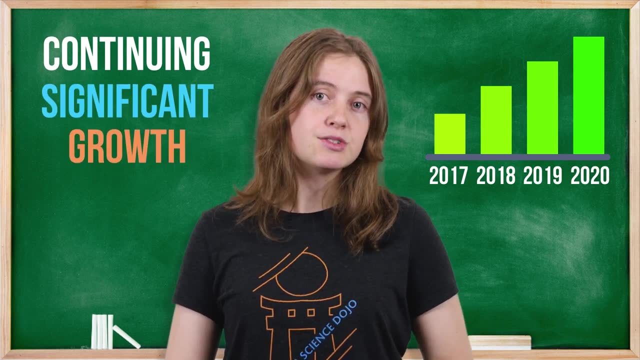 a million online users in the year ahead, significantly increasing from last year and even more so the year before then. When you reach a point of continuing significant growth, you might decide now's the right time to invest in better infrastructure for the year ahead and coming years. 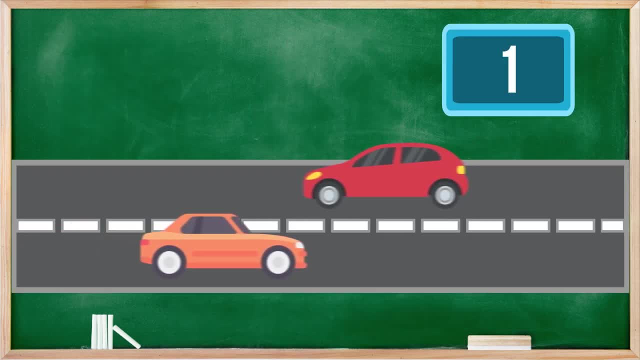 ahead. Another example is say you have a sensor device recording the number of vehicles that cross an intersection every 20 minutes. Another example is say you have a sensor device recording the number of vehicles that cross an intersection every 20 minutes. Another example is say you have a sensor device recording the number of vehicles that cross an intersection every 20 minutes. 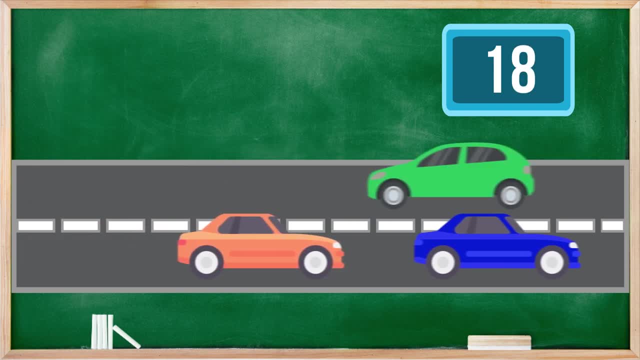 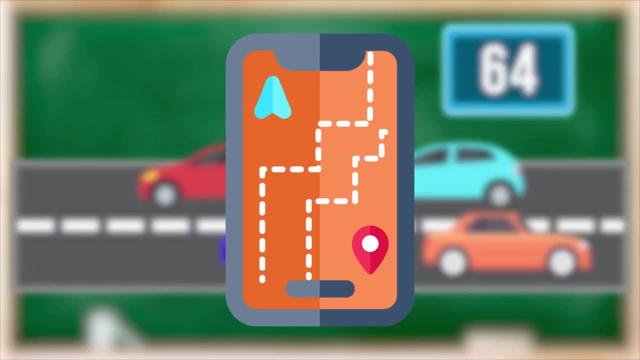 You could use these counts of vehicles to predict that in the next 20 minutes, traffic at the intersection is likely to spike to a huge amount. So now maybe your trip-laying app could reroute your drivers to avoid this congested, problematic intersection, distributing the traffic load more evenly across the roads. 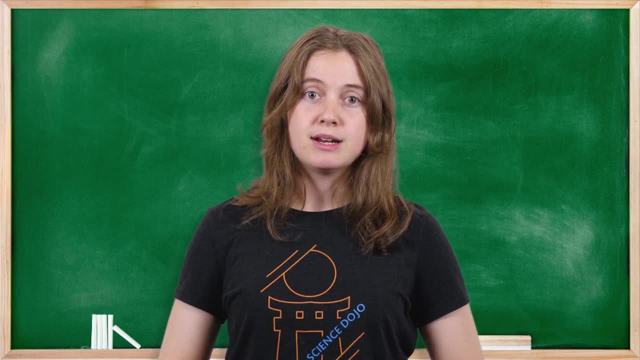 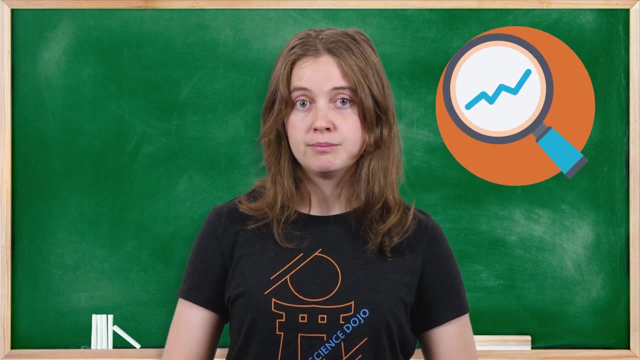 It is also possible to model data with no recognisable pattern or trend in time series. When there is a trend or pattern, you could look back at the whole of history of your data and see that the pattern occurred over time. But if there is no, 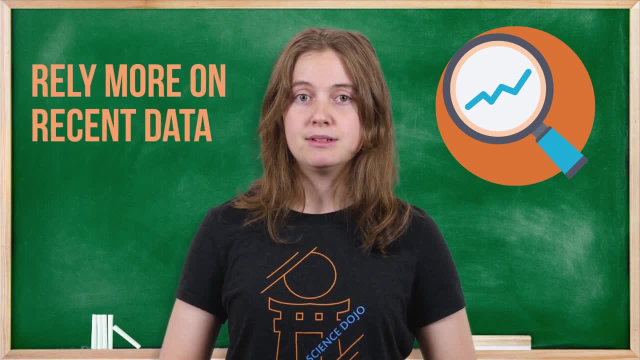 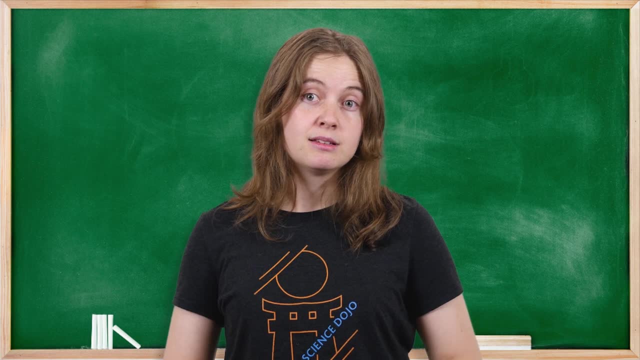 recognisable pattern, then your best bet is to rely more on what's recently happened and less on what's happened far in history. What's happened recently is more useful in guiding us to what will happen next than to look back at the whole of history, which only 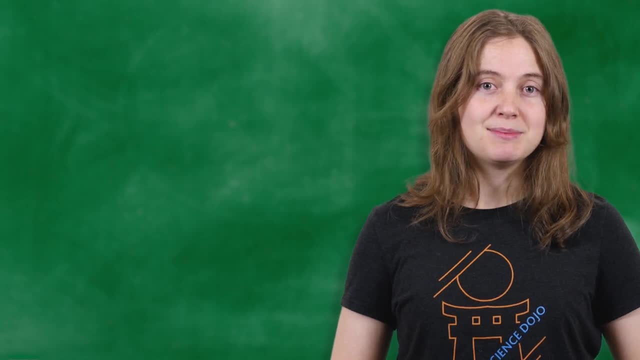 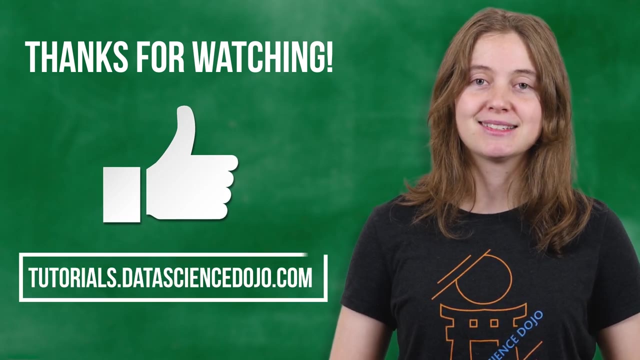 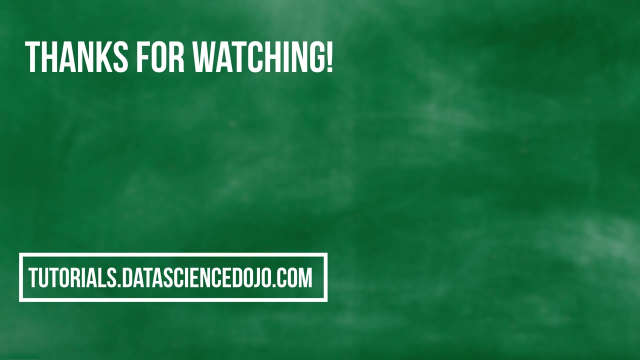 shows us pretty much anything could happen, And that sums up time series in no time. Thanks for watching. If you found this video useful, give us a like or you can check out our other videos at Data Science Dojo tutorials. If you have any questions or other problems, please post them in the comments below.